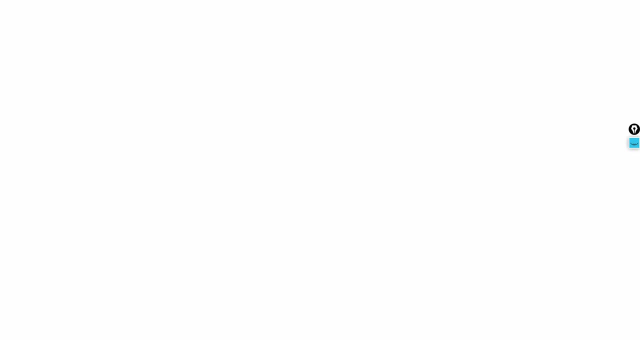 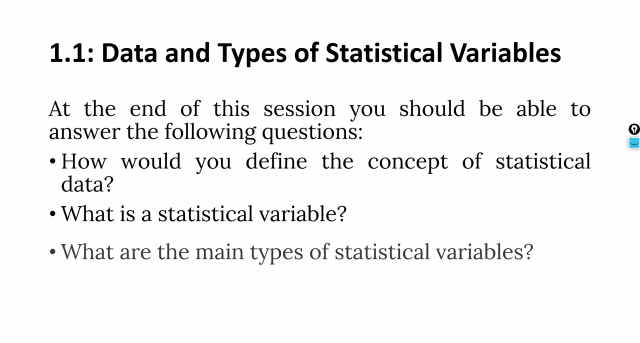 So the first step is exploring your data. At the end of this session, you should be able to understand or answer the following questions: How would you define the concept of statistical data? What is a statistical variable? What are the main types of statistical variables? 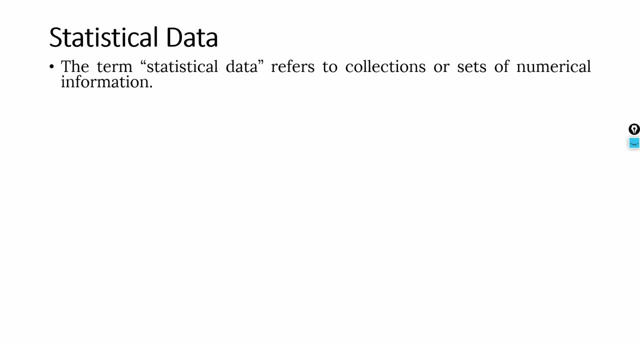 The term statistical data refers to the collection or sets of numerical information. Now, since we are focusing on statistics, obviously it has to be numbers. The information is located within cases or records of a separate individual, individual entities. We might have data based on years, let's say GDP per year, or we can have responses from: 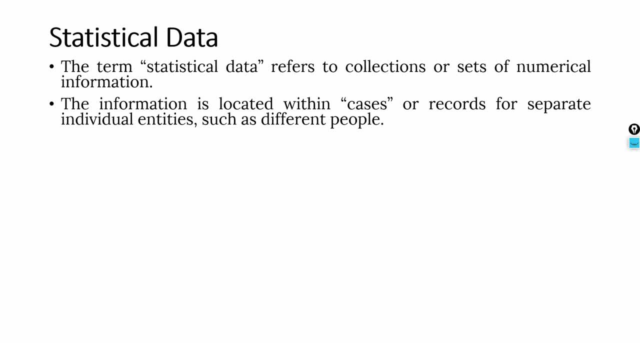 different people, So each response is a different case that is attributed to a particular respondent. However, cases can occur at multiple levels as well. Therefore, within data sets, you can have cases for different people, groups, larger entities like organizations or regions. 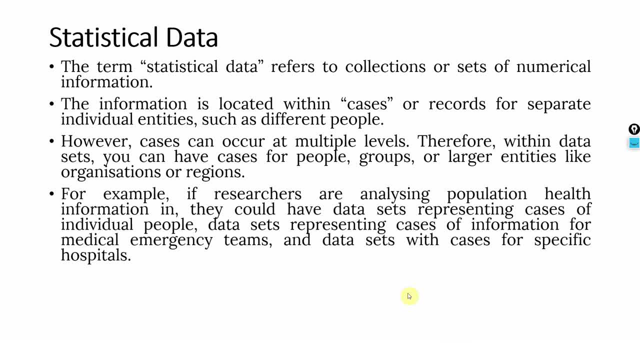 Now, for example, if a researcher is analyzing population of health information, they could have data sets representing. now you can have separate data set that represent cases of individual people. You can have data set representing cases of information for Medical Emergency Teams, or you can have data sets with cases for specific hospitals. 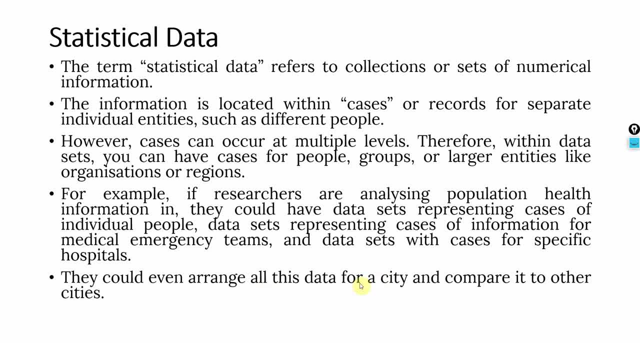 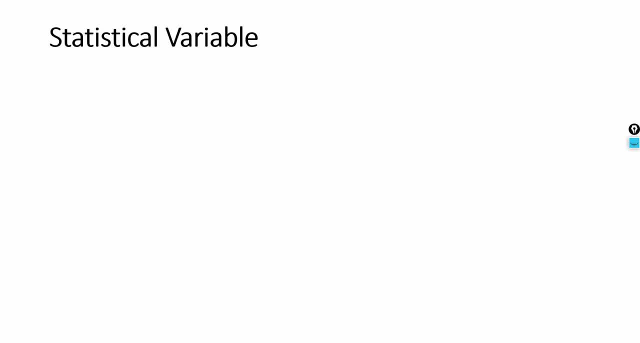 Now they could even arrange all this data for a city and compare it with another city. So that's the first step. Thank you as well. Now, what is a statistical variable? A statistical variable is a special type of mathematical variable. As with all mathematical variables, statistical variables represent a 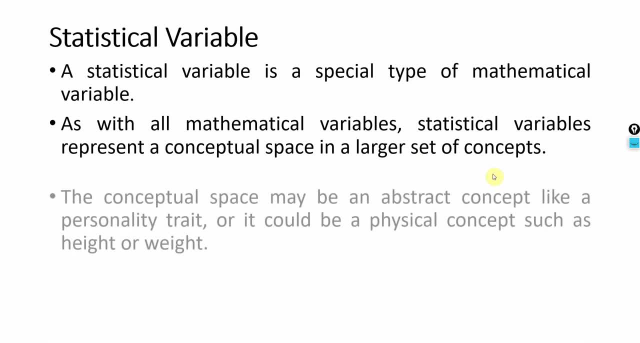 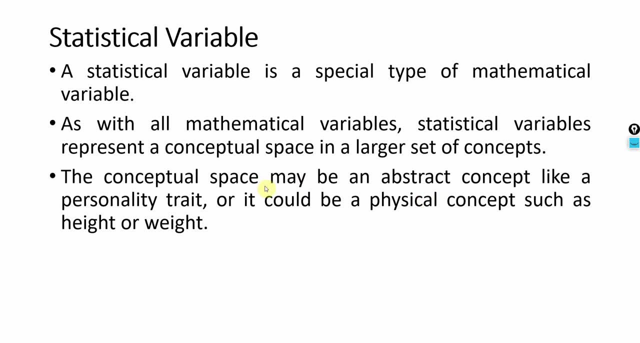 conceptual space in a larger set of concepts. Now that conceptual space may be an abstract concept, like a personality trait- someone is an introvert or an extrovert. Now that is, or that may be measured differently in different contexts. or it could be a physical concept, like height or 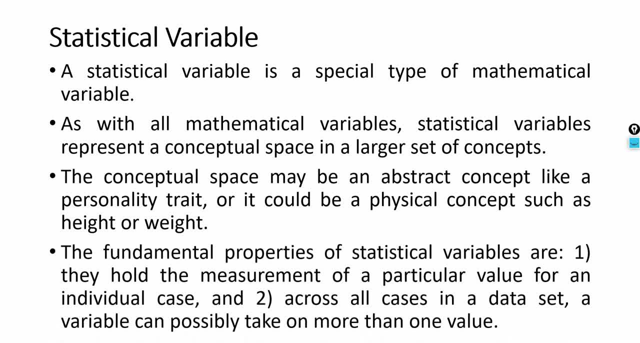 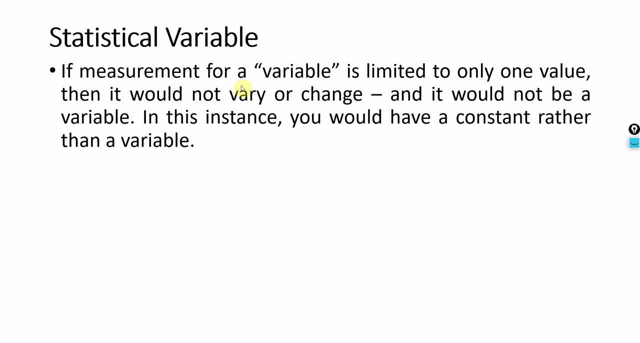 weight. that is visible. The fundamental properties of statistical variables are: one, they hold the measurement of a particular value for an individual case and, secondly, across all cases in the data set. a variable can possibly take one or more than one value. Now, if a measurement for a variable is limited to one value, now if a variable can only have one. 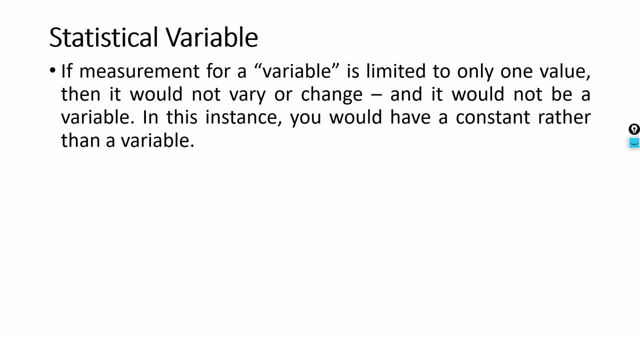 value and it does not change for a particular respondent or for a particular event, then it is a constant, it is not a variable. The value will change from person to person, from time to time, from place to place, and that is what makes a statistical variable variable: because it changes. 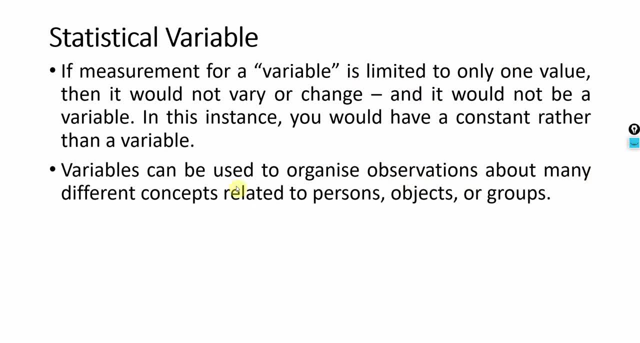 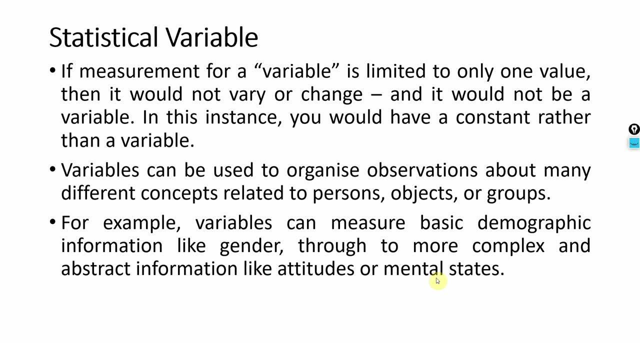 Now variables can be used to organize observations about many different concepts related to people, objects or groups. for examples, variables can measure basic demographic information, like gender- so gender is a variable- through to more complex and abstract information like attitudes or mental states, like job commitment, turnover, intention or perception. 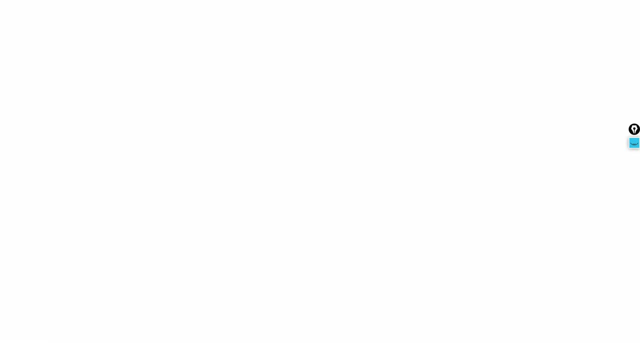 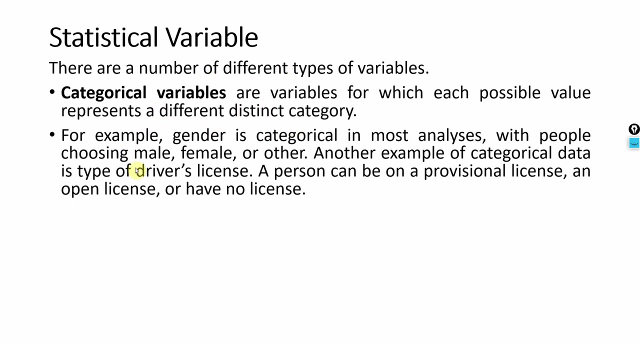 about the social responsibility of the organization. now, there are number of different types of variables. they could be categorical variables. now, these are the variables for which each possible value represents a distinct category, like gender, like job rank, like education. gender is a categorical variable. type of driver's license is a categorical variable. you can have a provisional. 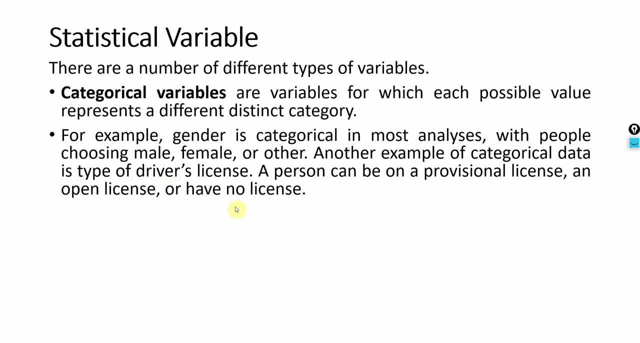 license, open license or you can have no license at all. city of residence is another categorical variable. it could be pishawa, london, la hore, mexico general government center or secure out source Manchester or New York. Now, in contrast to categorical variables, there are continuous 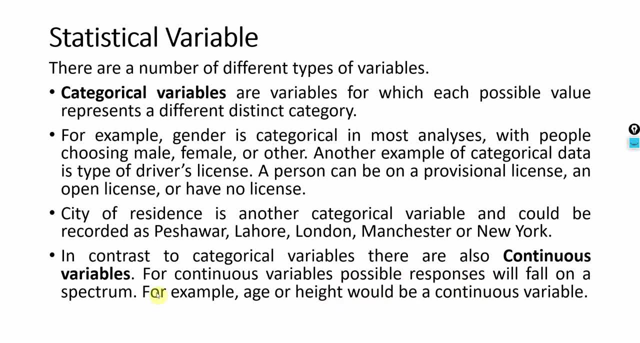 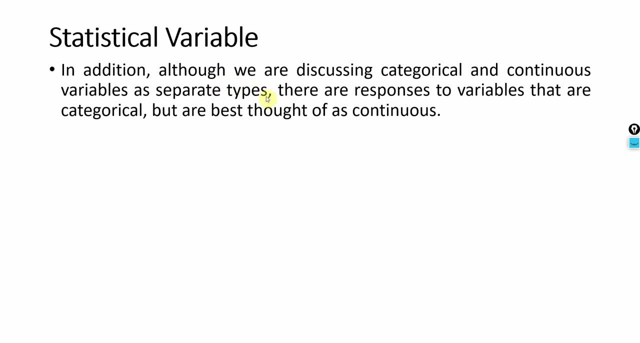 variables and continuous variables will fall on the spectrum. For example, age or height are continuous variables. Similarly, weight is a continuous variable as well. In addition, although we are discussing categorical and continuous variables as separate types, there are responses to variables that are categorical but are best thought of as continuous.